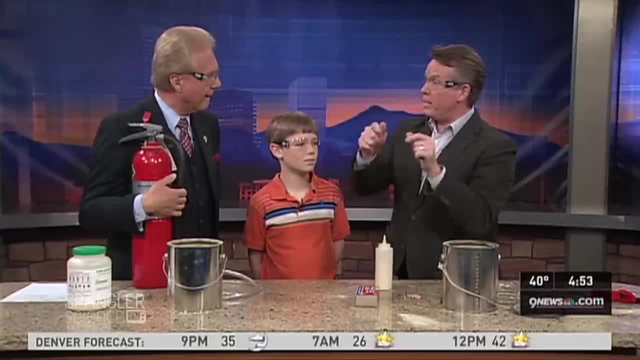 It's like taking a log and trying to catch that one thing on fire or bringing it up into kindling. So we've done this with a spore. This is a spore called lycopodium, and so special effects artists use it. 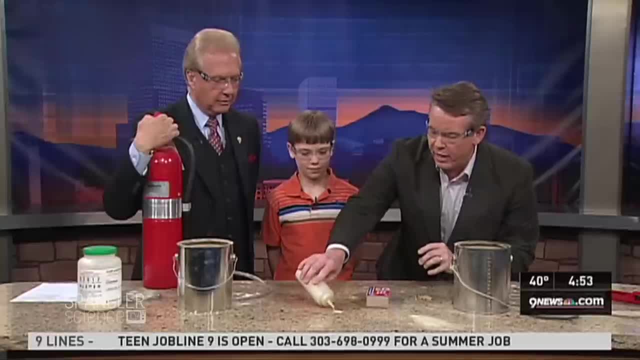 They use this a lot. So here is lycopodium. Oh man, So if I take a little bit of lycopodium and I put it here on the table and now I try to catch the lycopodium on fire, nothing happens at all. 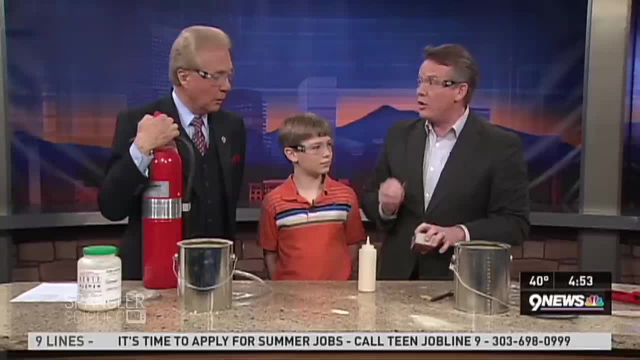 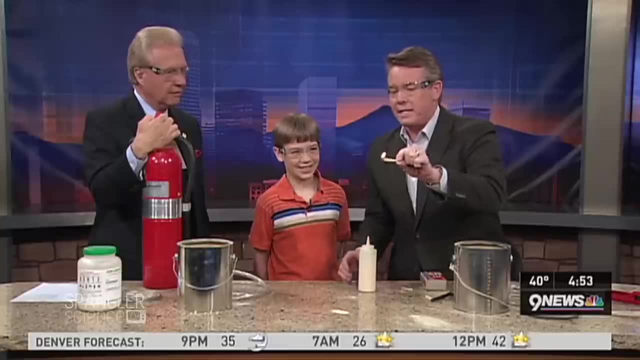 See, it doesn't catch on fire, But the moment you distribute it in the air, then you get something else, All right. so, Scotty, you got your safety glasses on, I do, All right. so one little piece catches the next one catches the next one. so it looks something like this: 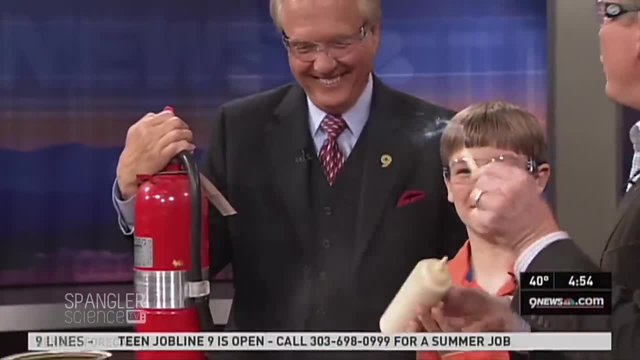 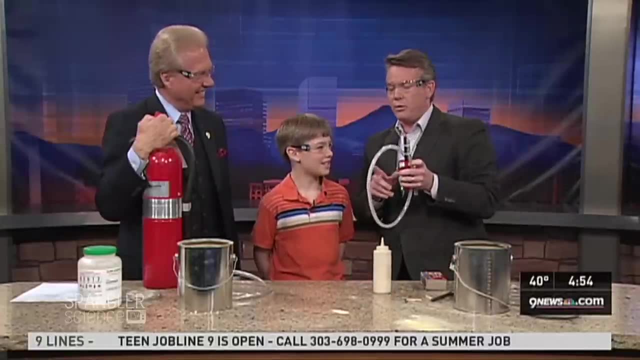 Here, watch what happens. Oh, Pretty amazing. see, Awesome, awesome. So, if you can imagine that release of energy Isn't that crazy. That was crazy, yes, I know, a little wild. So then I thought, well, there would be another way to distribute it. so I learned this from a special effects artist: 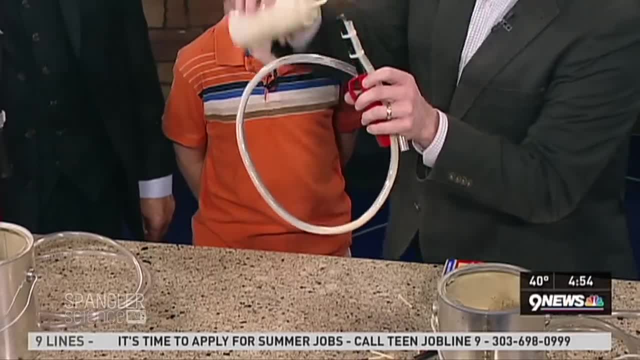 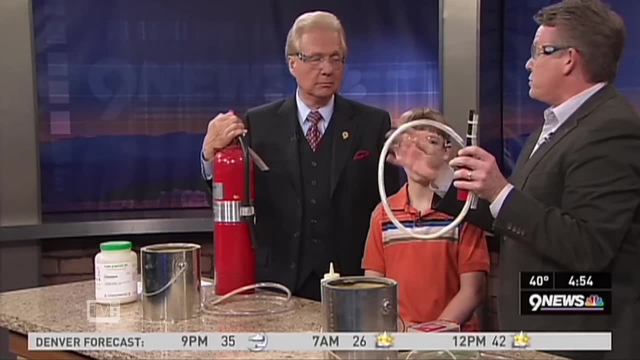 So this kind of goes in here like this. So here's our lycopodium that goes in here. So again, the real danger is the fact that it's distributed in the air And once the little grain, if you can imagine, a grain elevator. here's why it exploded. 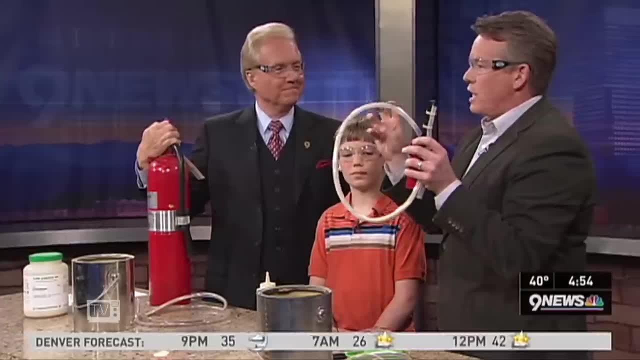 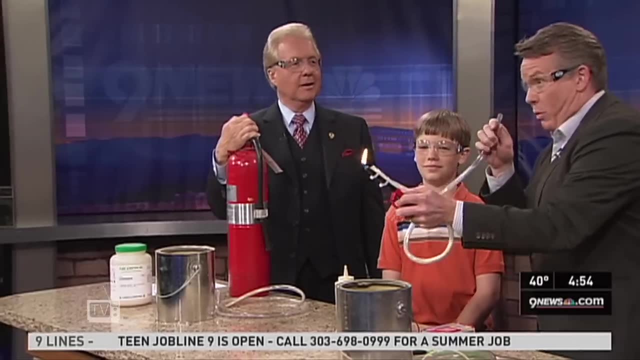 Imagine a grain elevator not having good ventilation. back then, If a spark at all sets something off, one catches the next. so it's a chain reaction. If you saw this in slow motion it would be pretty crazy, But here, watch this. 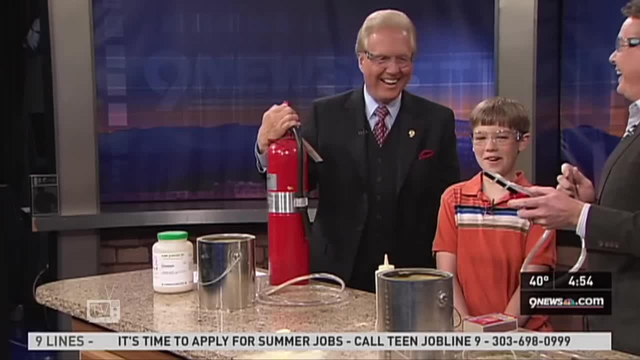 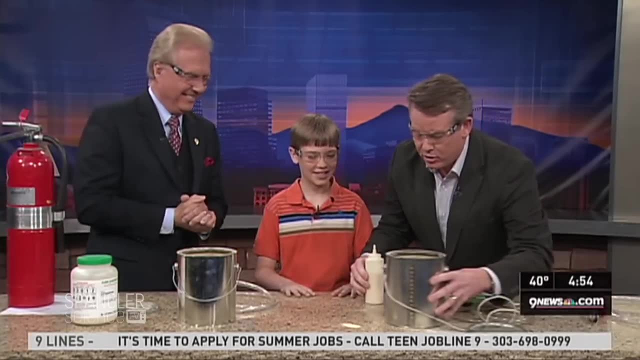 I'll do it right to the camera Watch. Oh, Isn't that wild, It goes, That is great. But then we thought: you know what? why don't we recreate the grain elevator, right? Why not? Yes, All right. so here's what we have here. 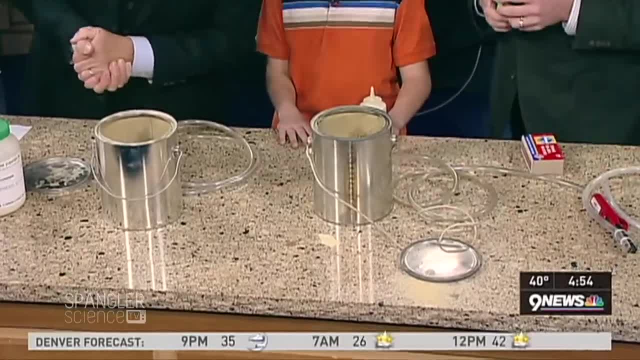 So, Mr Koprik, look down inside You can see we've got some candles inside the can. Yes, we do Got it. Yes, So I'm going to light these on fire here like this, All right, So there's no problem with that. 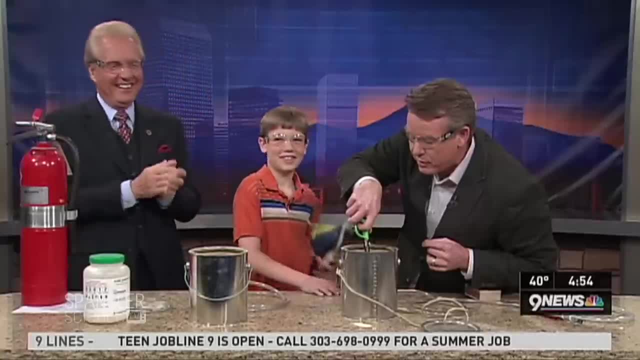 Hey, Scotty, give me your shoe. I need your shoe, buddy. Okay, Okay, got that, So I need your shoe. Got it All right? so, just in case, I'm just lighting this on fire, so we just have a little. 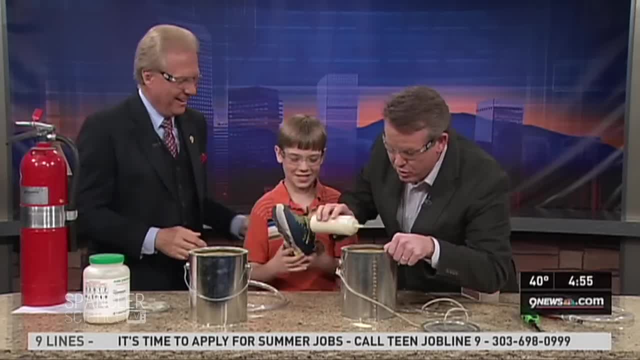 Oh yeah, that's going to be good, All right. so now I think we've put: This is not an advertisement. No, no, it's not an advertisement, It's good. So you see, we're putting it like a podium inside there. 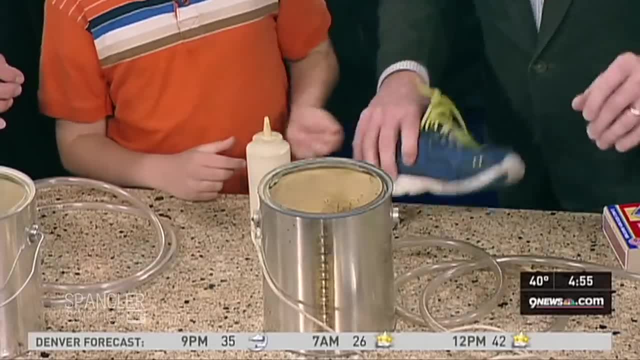 Oh, that was close. Be careful, Be careful, We're fine. Okay, got it, Yes, Okay, feeling good. So now this goes on here like this, Okay, And we kind of push it down Like the grain elevator.